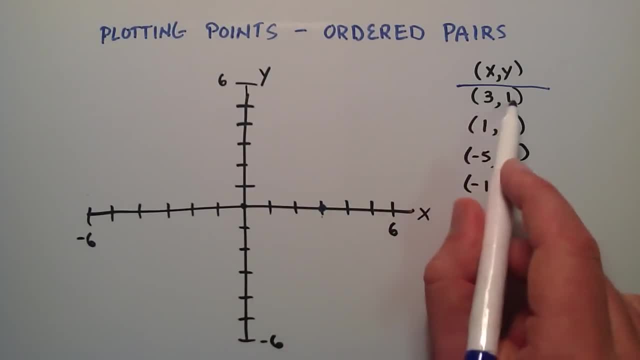 Puts us right here. So that's our x component of this point. right here. So we need our y component next. So our y component is 1.. So once again, we start at the origin and we go up 1 unit in the y direction. 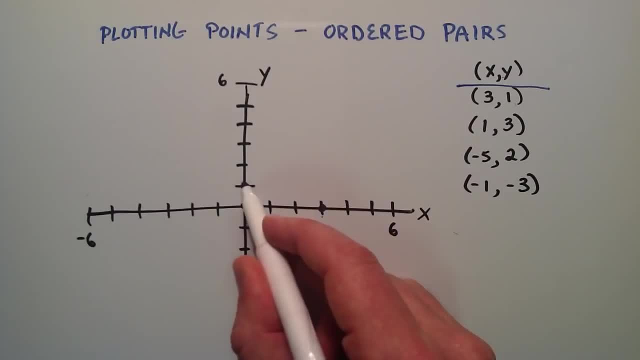 This time, since it's the y component. So up 1 unit in the y direction puts us here, And then we just draw our projections off of those two components, And where those projections cross is going to be the point represented by this ordered pair. 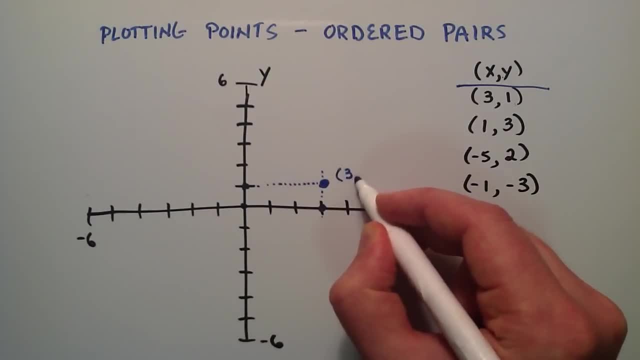 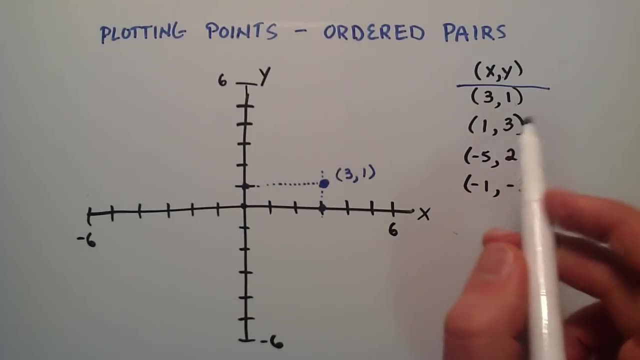 So this is the point represented by the ordered pair: 3, 1.. So now let's look at 1, 3.. So it's really the same information, except for we've switched the x and the y values. So when x is 1, when our x component is 1, we simply go over from the origin 1 unit in the x direction, this time. 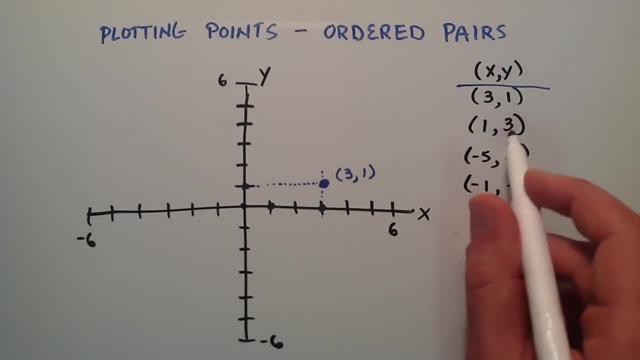 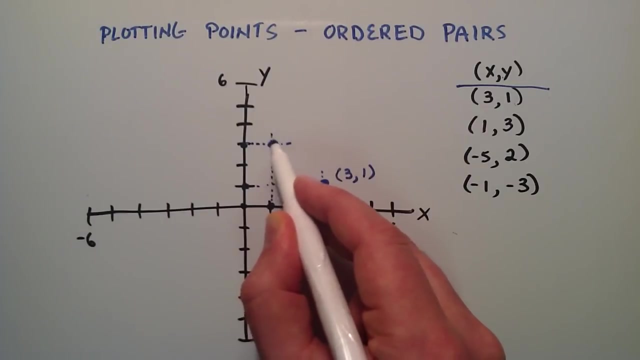 And our y component is y. so we go up 3 units in the y direction, So that's 0,, 1,, 2, 3 in the y direction, And then we just draw our projections here And then where these two projections cross would be our points, represented by the ordered pair. 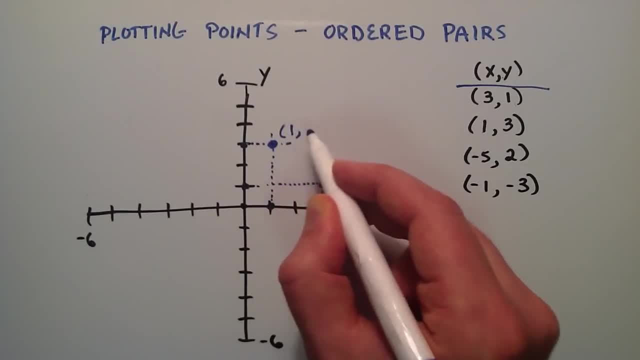 So this is the point represented by the ordered pair 1, 3.. So let's go ahead and do these two now. So this one right. here we have an x component of negative 5. So, starting at the origin and going on the x axis in the negative direction, 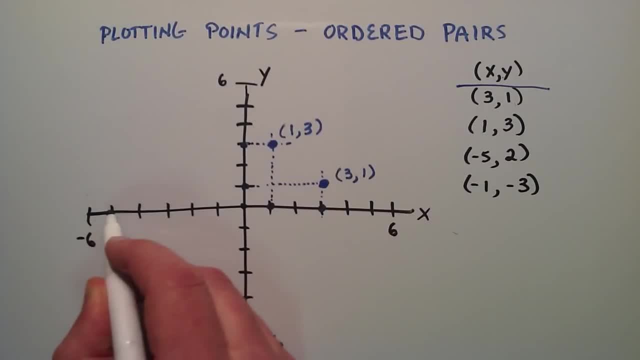 Negative 1, negative 2, negative 3, negative 4, negative 5 puts us here for our x component And then our y component of this point is 2.. It's the y component. So we start at the origin once again. 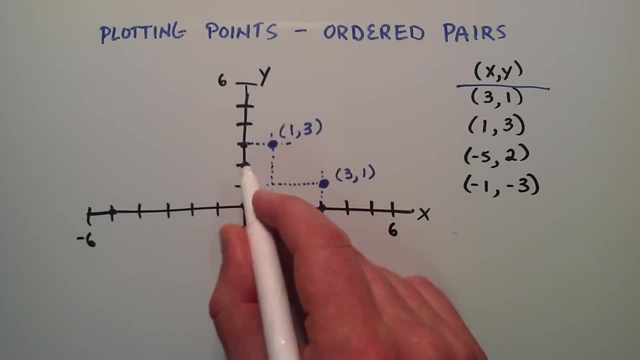 And then we go up 1, 2 units in the y direction on the y axis here, And so then we just draw our projections once again, And then the other one comes off of here, And so where these two cross is going to be the ordered pair: negative 5, 2.. 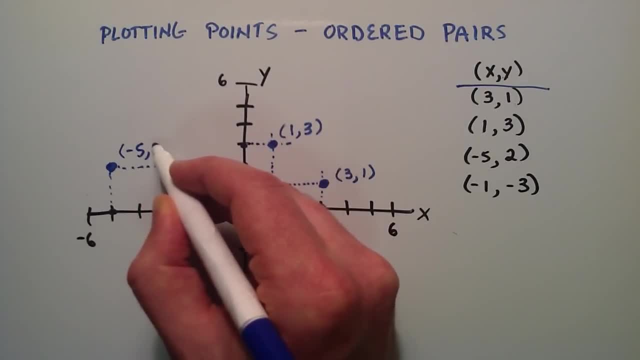 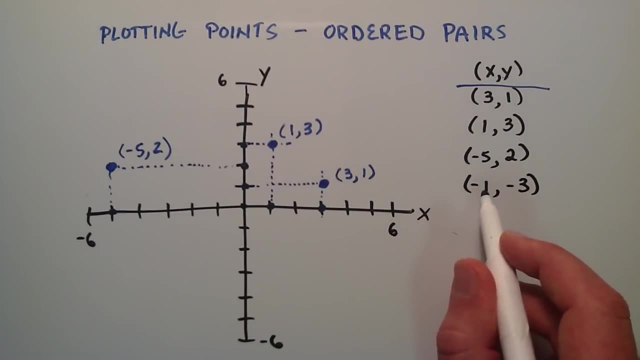 So that's the point represented by the ordered pair: negative 5, 2.. And let's go ahead and just do this one now. So x, our x component, Is negative 1 for this point. So on the x axis we go over negative 1.. 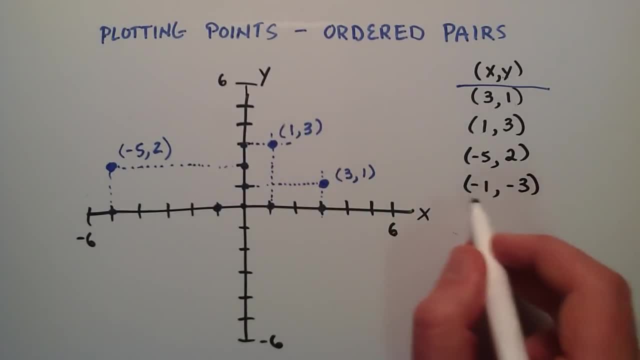 So that puts us here. And then our y component for this point is negative 3.. That's the y component. So we start at the origin, Go down 1,, 2, 3 units in the negative y direction, negative 3.. 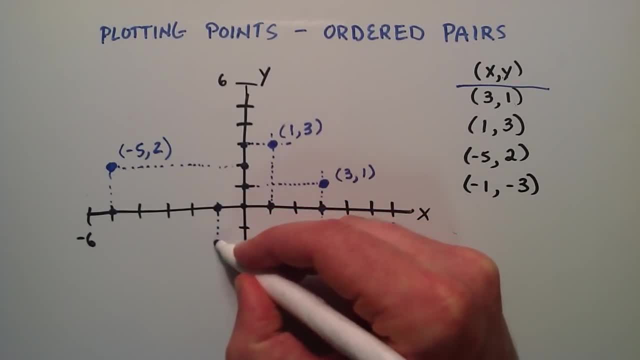 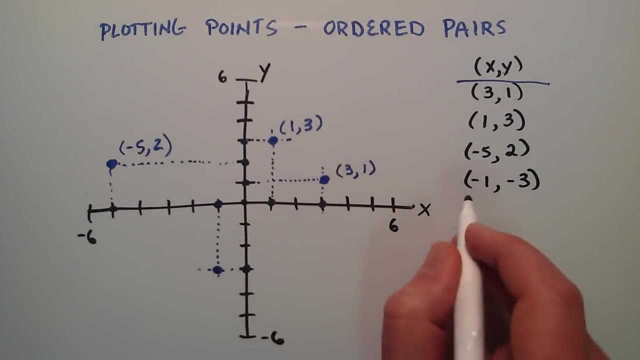 And that puts us right here. So then we just draw our projections off of those two as well, And where those cross is our point. That is right here And that is represented by the ordered pair negative 1, negative 3.. So negative 1, negative 3 is the ordered pair that represents this point. 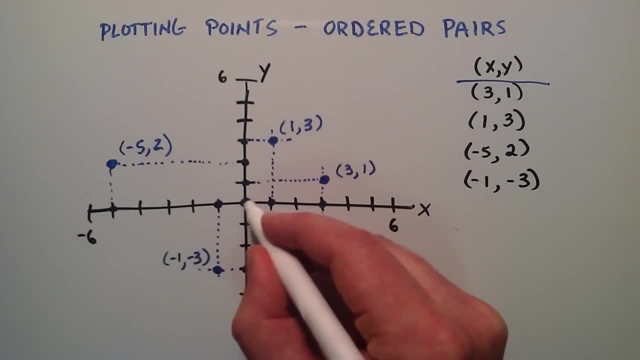 And I guess one other thing I could point out right here: The origin we can also represent by an ordered pair. So the origin is just simply the ordered pair: 0, 0.. 0 on the x axis, 0 on the y axis. 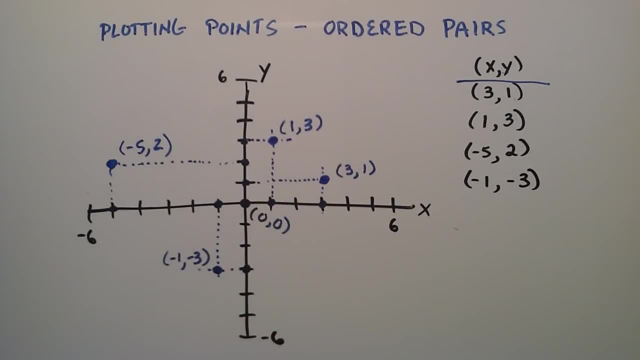 That's the origin. So anyway, that was some examples on how to plot points on the x- y coordinate system By looking at the values of their ordered pairs. So thanks you guys for watching And we'll see you guys in the next tutorial. 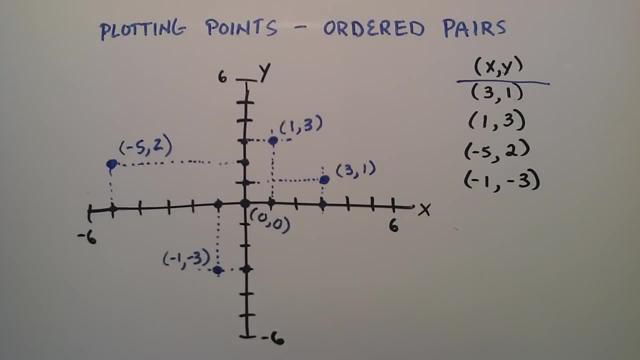 Have an excellent day And if you haven't already, don't forget to subscribe.